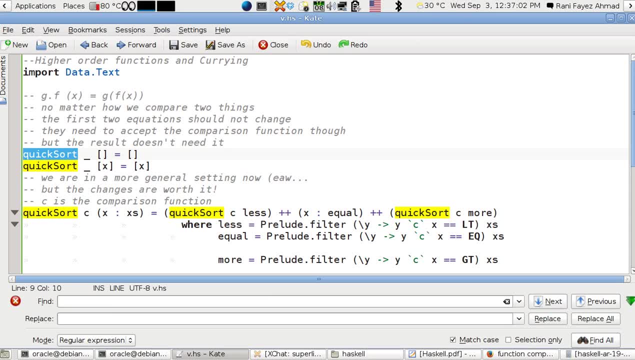 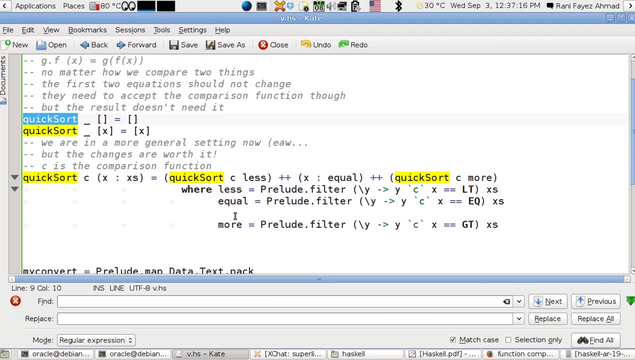 seen this function- your university- you know how hard it was for you to write it in C or in Java, and you know recursion usually is hard in C and Java. so if you see it here in Haskell, just those six lines and you're done. okay, whatever they are. so this is how the function is done. 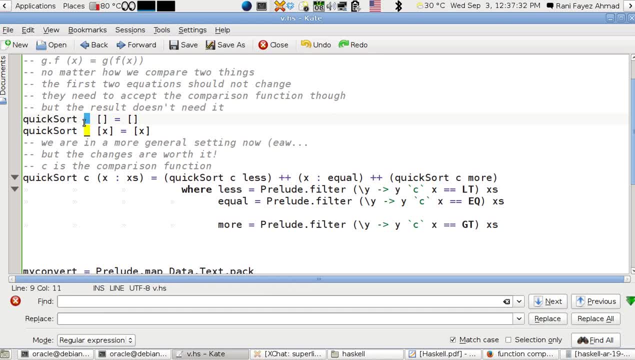 it starts with the function, of course, quick sort. then here there is any function, okay, which you use it to compare where things are. okay, I'll explain a bit for those who don't know. okay, with respect to the point, or with respect to that number. okay, that you want to start with to reorder things. 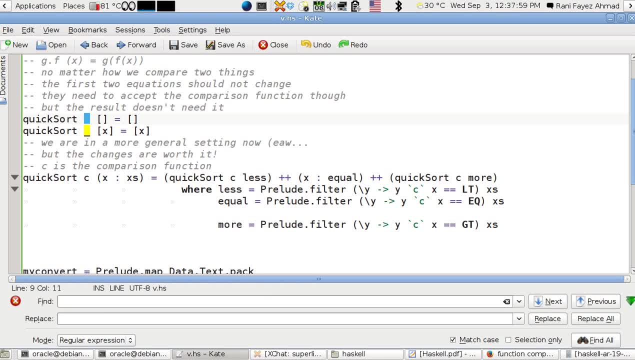 according to it, okay, whether it's before it or after it, okay. and if, if you are ordering here, as an input, an empty list, of course it should give you an empty list, okay. next, if you have a function that you're going to use to compare, okay, and you've got just a single singleton list, okay, it just has. 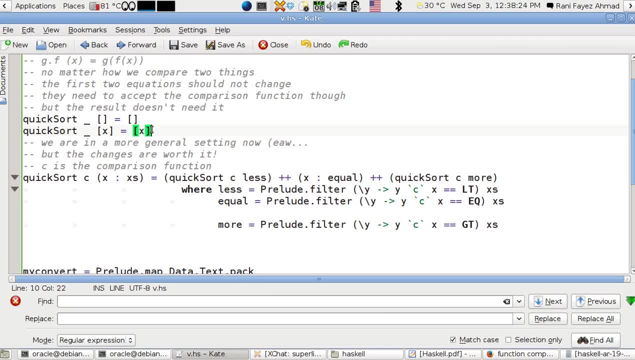 one element. it will give you that singleton. okay. now let's say I have a full list, a complete list, okay, and I wanna a quick sorted. see, this is our part where the real quick sorting goes. now, C represents the function that I want to use to compare now. this function should be of: 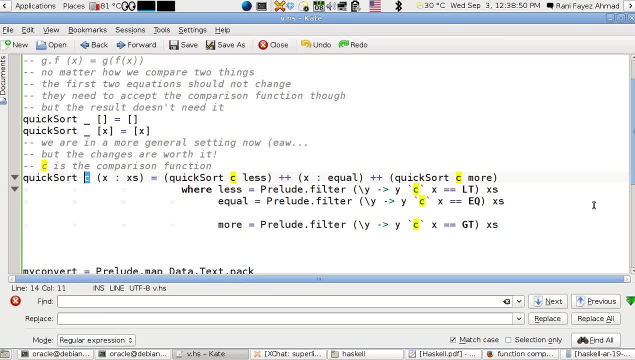 the type or okay, which means order, which means ordering, which should give me, whether, as a result, LTE for less than, okay, or equality, for you know, equal, equal, equal to between two final two members, okay, and the greater than- if it is greater than, of course, okay if it gives me that the comparison is greater than now. so, if I 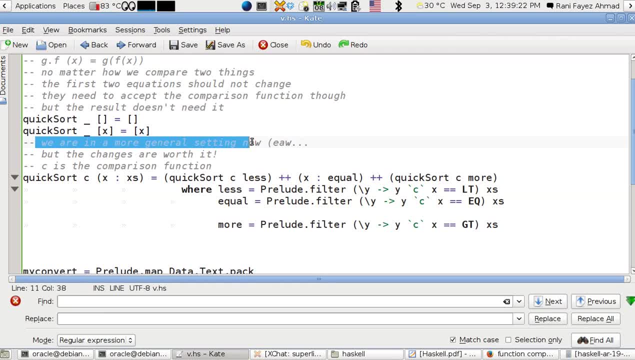 take, for example- let's start with an example here- this thing okay, and we start with, of course, the letter W. okay as the starting point. now you take everything that's before the W, like a and e. you put them before the W, to the left of the. 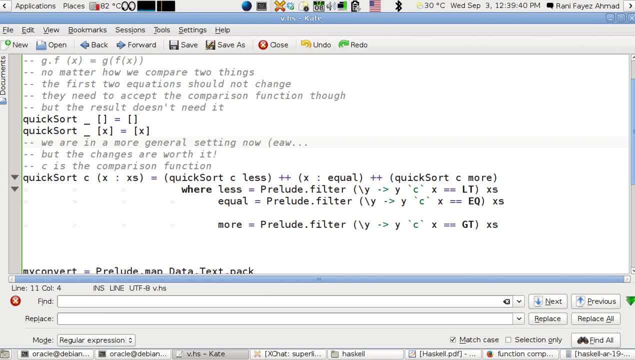 screen, okay, and the things like X, Y, Z: okay, put them to the right of the screen. okay, just put them randomly. don't care about the order yet. okay, this is the first step, only, okay, so. so what will happen? I'll get according to the part of the thing. okay, I'll get either. now let's see. here we go until like: 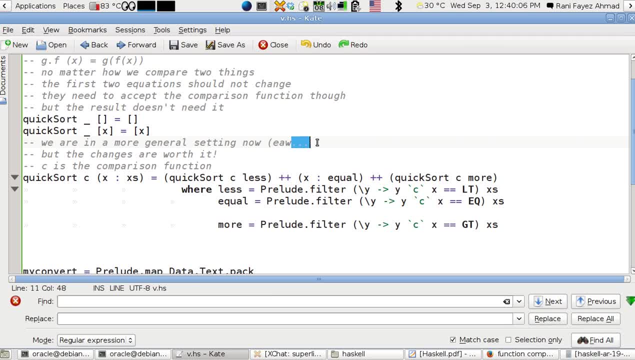 okay, and we take this one here. you can move away whenever you or we can again put on from the right. so when we put on to the left, like I said above, okay, we will get this w we'll put a cut in the middle here in between. okay, let's get. 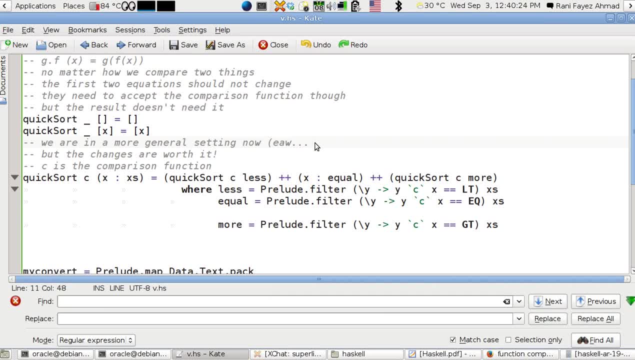 started. let's start moving the walls. okay, it will start standing. it's going to and get it sorted again. okay, why? because, if you look here, I'm calling quicksort on the same comparator. okay, with the parts which are less and what's less, I'm using the prelude filter. 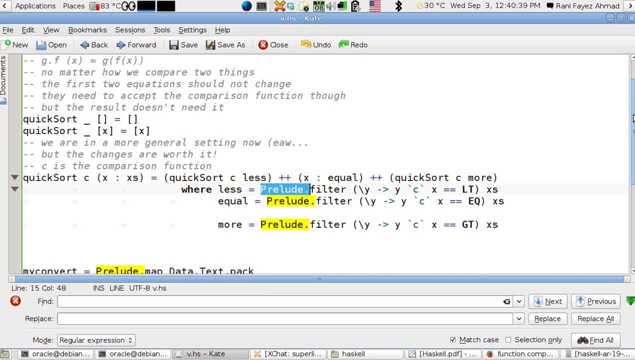 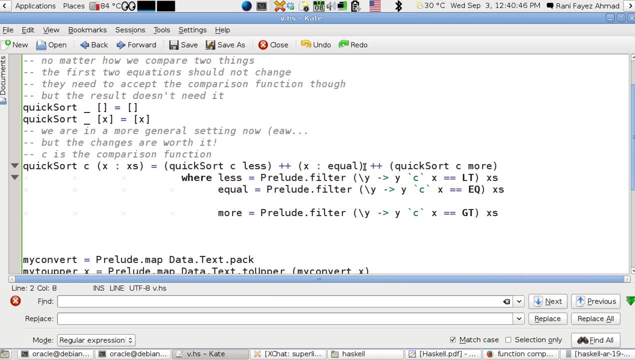 because there's a filter function inside the text class here, okay, the text part here, okay. so I'm just using the very basic filter that comes from Haskell, okay. and because I'm using things which are, which which tell me that they are less than it will filter them out and gives. 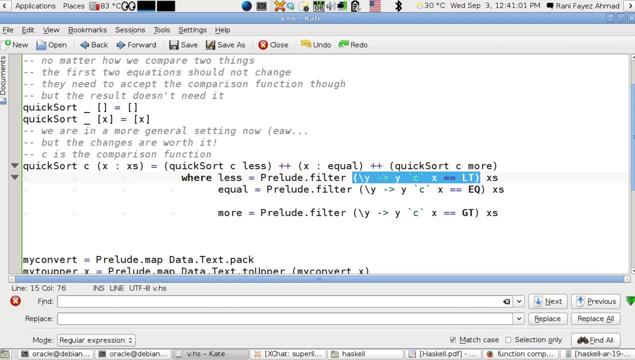 me, those which are lesser than X and the rest of the string. okay, or the less, the rest of the list, okay. so you'll be left out with the things that are bigger than and equal. okay, and on the next, on the equal part: okay, we just left with the things which are equal. okay, but you don't touch. 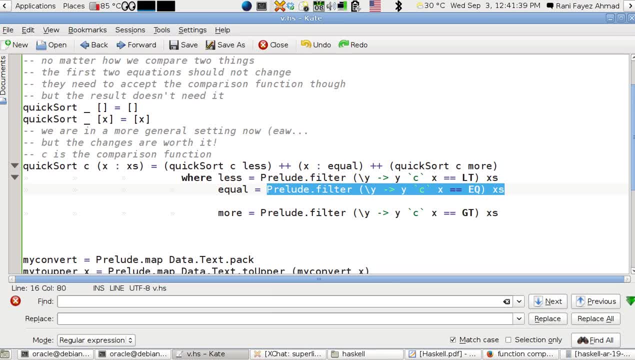 the things which are, yeah, I mean you take the things which are equal and you leave the things which are greater and less than, and similarly here with the greater than, okay, just take the greater than, and if the less than and equal, okay. now you take always the less than and the more, okay. and 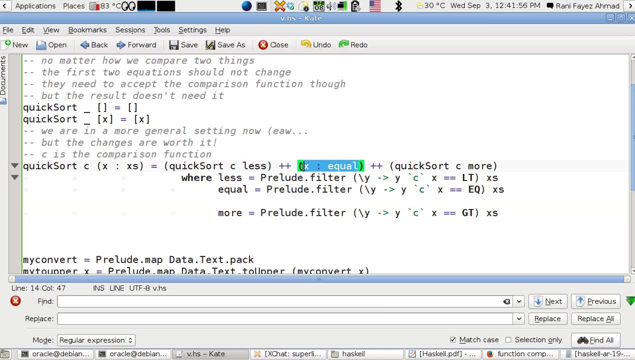 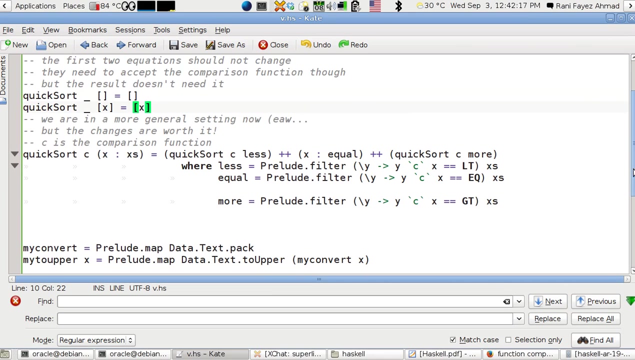 the less of the equal is always constant in the list, okay. and every time you call quick sort on the list and quick sort on the more and you get a tree like structure, okay, until you finish and reach this uh starting point, okay, or this base case- cool. so it will all the time recurs. 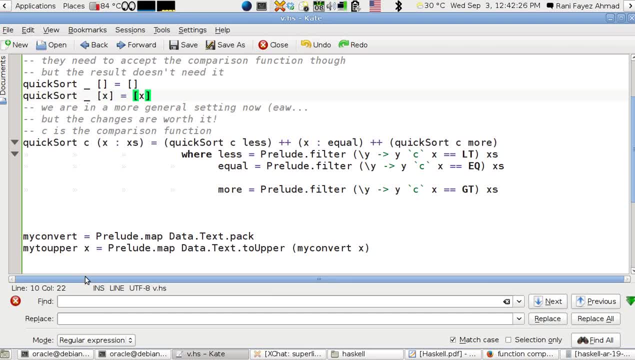 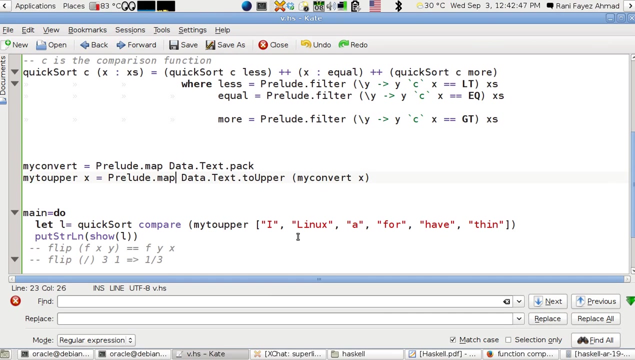 um, what's occurring now? carrying is when I say, for example, I want to use to upper from the data dot text, okay and uh, I want to use the prelude here, dot map. okay, so I can map every word in that list. okay, for example, I have this list, okay, I Linux a and I want to make it all uppercase cool. 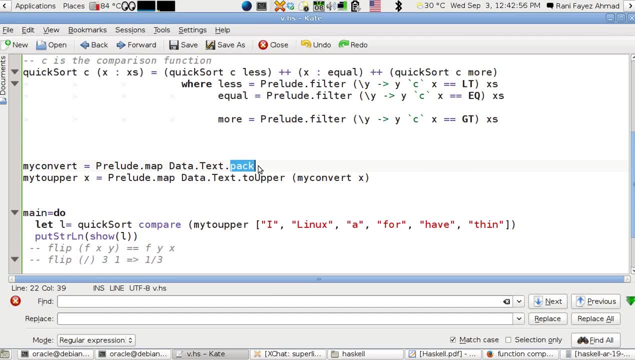 so the datatxtpack should uh like, by definition, it should turn the type string to the type text. okay, this is something required just to do a whole string. uh, uh, conversion to upper or to lower. you can also use the taller to lower. now, what concerns us about the cutting is that, if I want to uh make 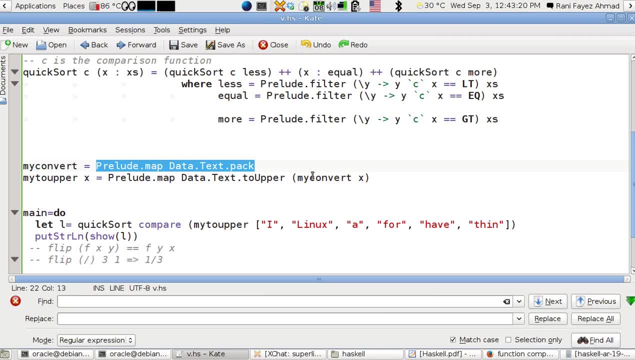 a summary of those. okay was like: if I want to use them here instead of my convert, okay, like an alias, okay, so I could have used this way. so, uh, it can automatically Haskell know that has to come to pass X to the rest, so as if you made an alias to my convert word. okay, and therefore here: 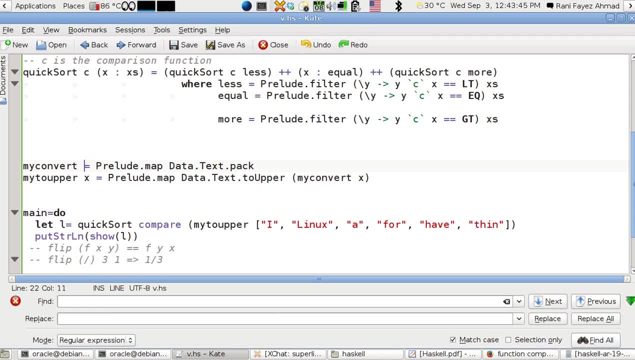 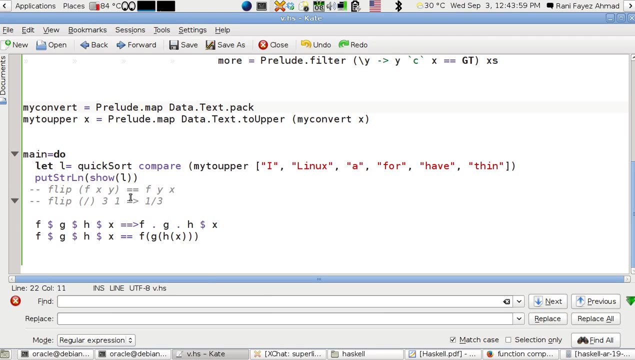 you get an X, okay, it will know by itself that has to put the rest of the parameters. okay, this is another thing in Haskell. okay, uh, we can uh do is, uh, if I have, if I want to use this function called flip, okay, uh, and this function takes a another function with two parameters. okay, now, uh, this: